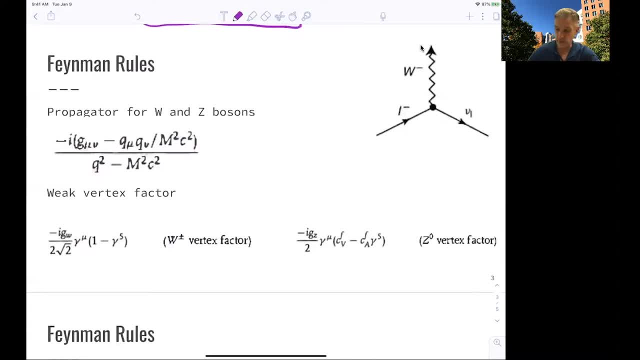 in order to get moving. So we can, for example, look at this vertex here or this point here, This component of a Feynman diagram And what we need to analyze. this is the propagator for the W and Z boson and the vertex vector. So this vertex vector now looks a little bit. 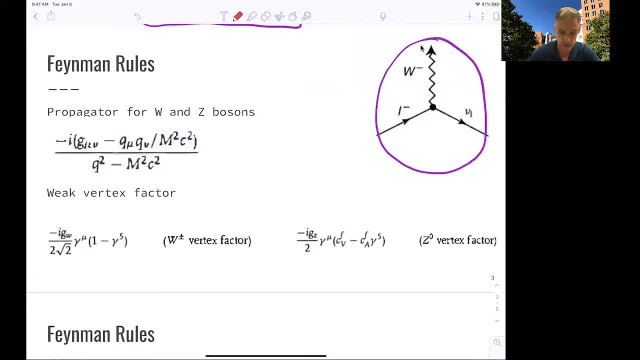 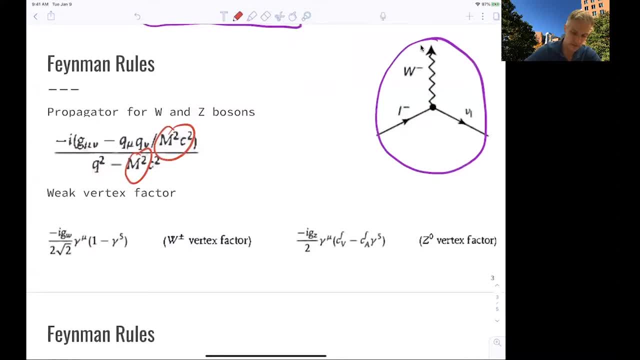 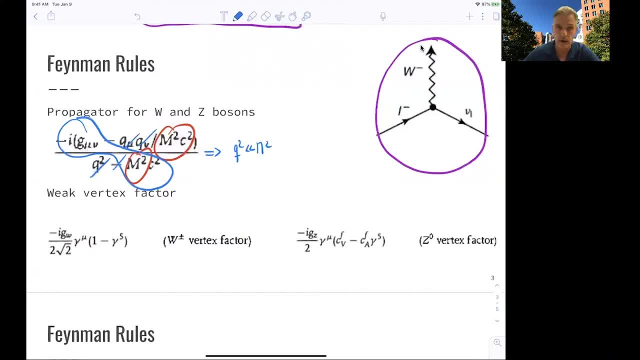 vertex factor which looks similar to the one we have in QED. However, there's no 1, but just in 1 over m squared term, which is constant. So we would see that we can describe this in the context of the Fermi theory, which 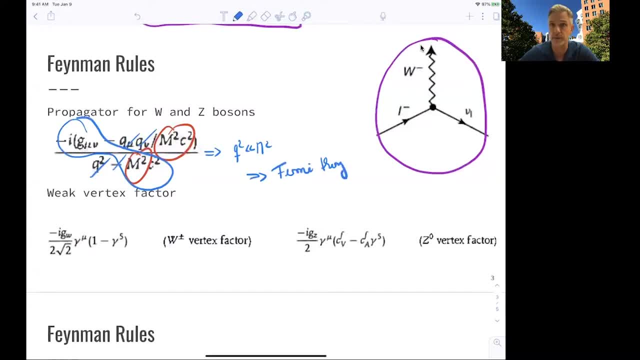 is a low energy approximation of the full theory of weak interaction. It's kind of an interesting concept and it extends to the entire understanding of the standard model. It might be that our standard model, when we have all the packages together, describes a lower energy approximation. 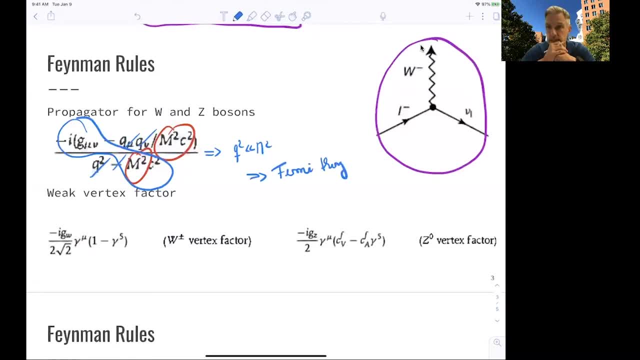 of a more holistic theory which we then can discuss under the concept of a grand unified theory, maybe with a symmetry group which is embedding the symmetry groups we need for QED, QCD and the weak interaction. All right, but that's a side remark. 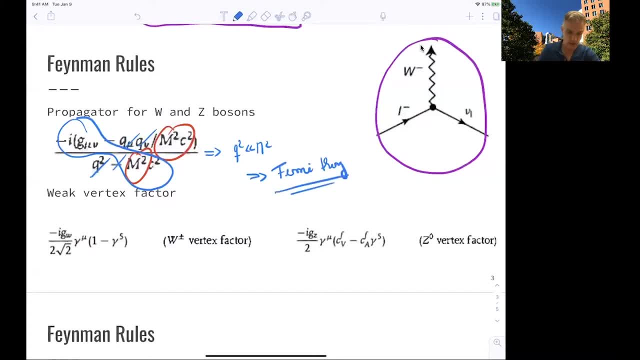 So we look at the Fermi theory a little bit more later. The vertex factor itself: I'm describing the vertex here. It's given here for the w boson and also for the z boson And it looks a little bit more complicated. 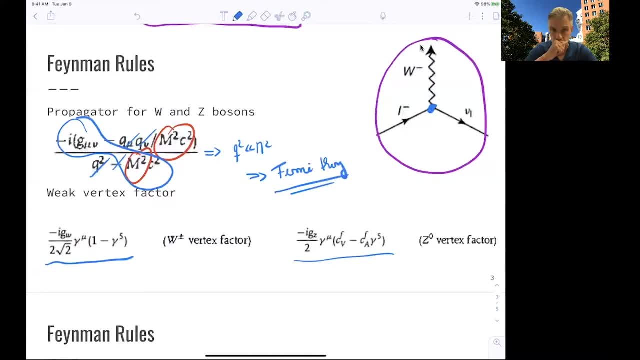 than the vertex factors we have seen so far. So what you notice is that there is a parameter which is associated to the strength of the interaction and the gamma matrix, But there's also this term here which has two components: There's a 1, and there's a gamma phi. 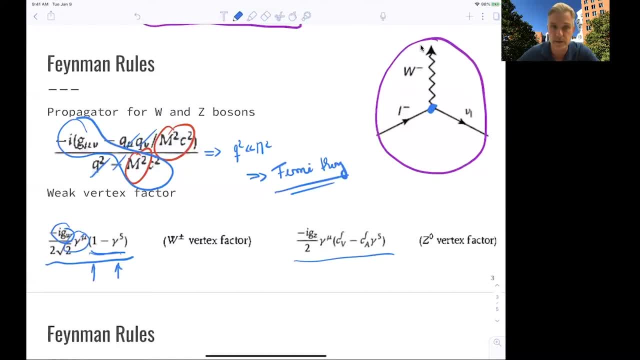 All right, we have talked about gamma phi matrix already. We can later identify those as individual currents, coupling to vector current and an extra current. So this looks even more complicated. now for the z boson, because here we have not just numbers of 1,. 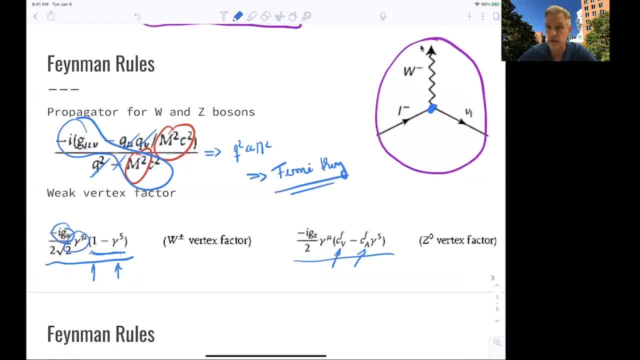 but an additional factor. This factor, cv, is a vector. It's a vector, It's a vector, It's a vector coupling And it's specific for each fermion. So each fermion has one of those constants And there's a second part of a package or set of constants. 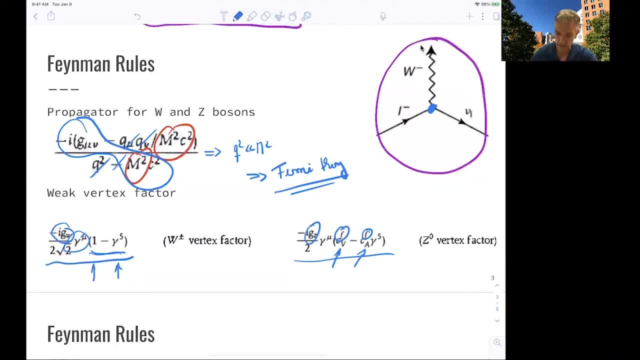 for the axial current. You have a second parameter here, which is the strength of the coupling of the z boson. So at this point we just take this book rounded and we can do our calculations. And on the next slide I'm going to explain to you. 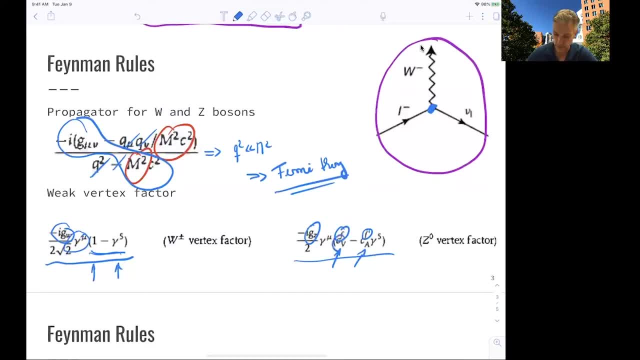 what the corresponding numbers are, what the values are for those parameters, cv and ca. Later we will see how it comes to this more complicated structure and why there is a vector and why there is an axial current in the weak interaction. 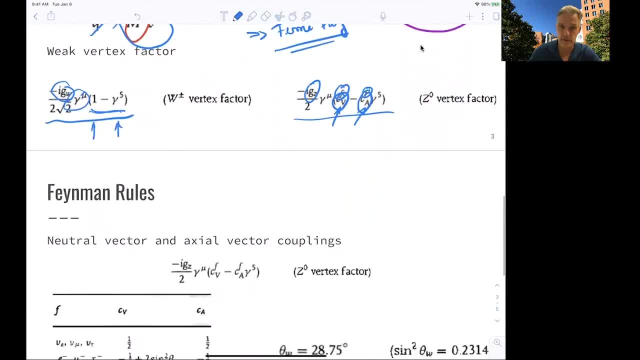 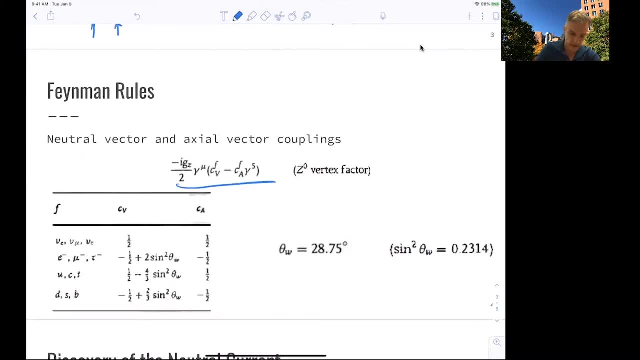 But for now we just take this book rounded and we just take this as a recipe. So now for the neutral. so we just have seen that this is the vertex vector, And here for all fermions, we list what these values are for cv and ca. 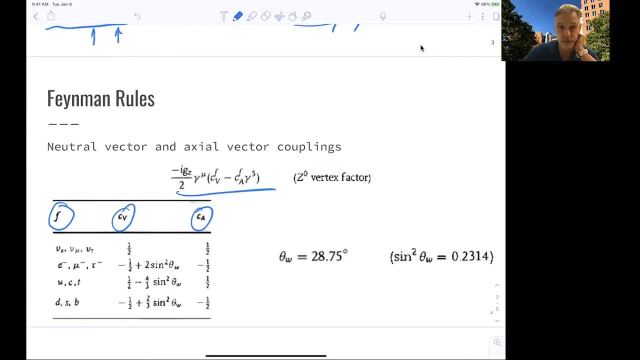 What you can see is OK. for the neutrinos the factor is 1 half, both for cv and for ca, And for the charged leptons and quarks there is an even more complicated term here which includes a new parameter: sine square theta w. 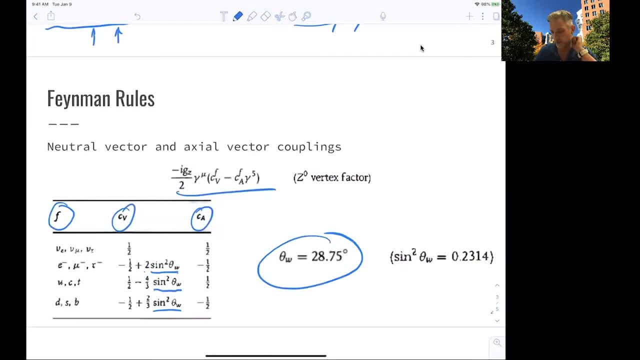 The value of this is 28 degrees Sine square, theta w is 0.231.. OK, OK, OK, OK, OK, OK, As a little bit of a preview here already, the fact that there is a new parameter and an angle involved. 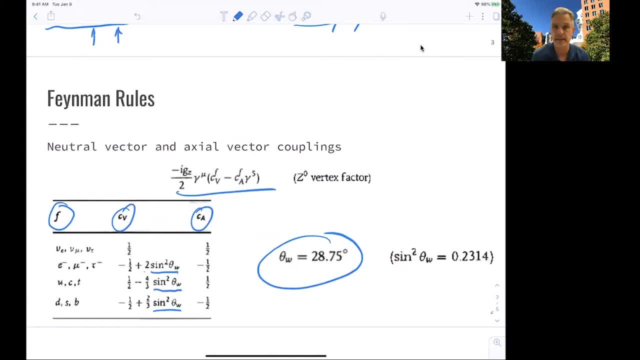 leads to, or can be explained later, by the fact that the weak interaction is actually a result of a mixing between an original weak interaction and QED, So there is a mixing going on. In other words, the Z boson itself is a mixture between the sine square, theta w and ca. 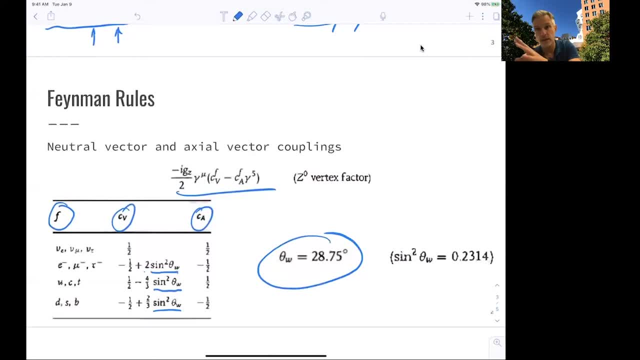 In other words, the Z boson itself is a mixture between the thing which couples to the weak part of the particle and the part which couples to the electrically charged part of the particle. And you see that that's why there is a very simple factor for the neutrinos who 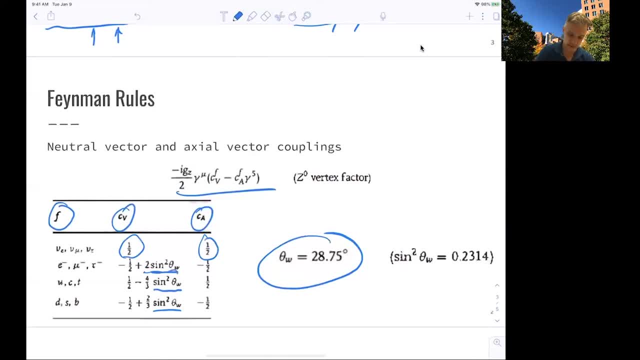 are electrically neutral and a more complicated term here for the electrically charged particles. And you see that this is the electric charge here, or two times the electric charge of the particles. OK, OK, OK, OK, OK, OK. 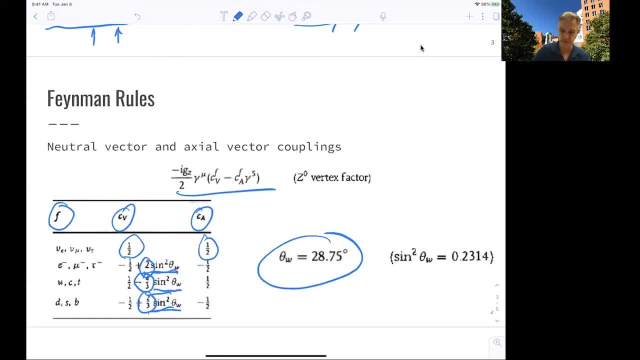 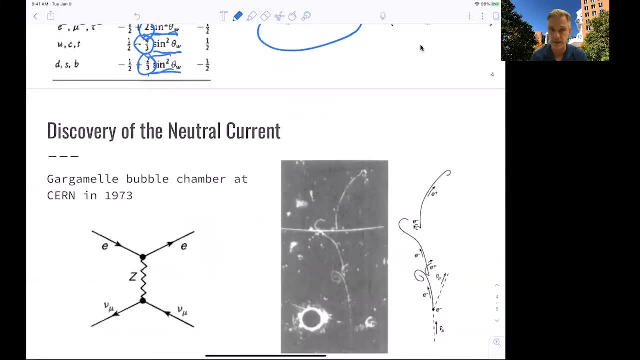 But for now those are all just constants and recipes to be used. One additional word on the history of the neutral charge, of the neutral weak current, is given here. So in the 60s and 70s the standard model was slowly developed, a little bit more slowly. 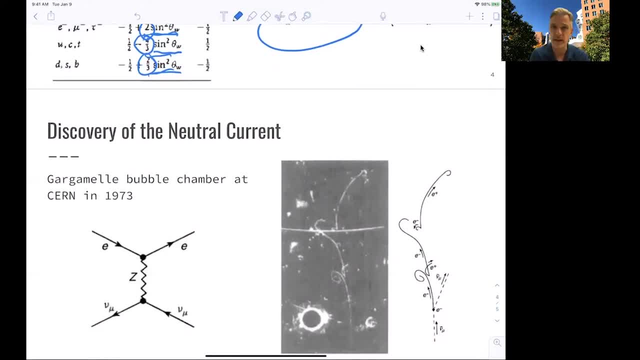 than we do in this class, And there was an hypothesis that there has to be something like a neutral current somewhere, but it has never been observed in nature, And so with bubble chambers, specifically the one at CERN, one was able to actually see those. 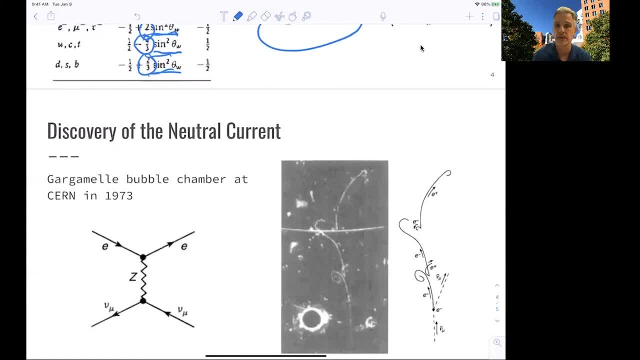 see, virtually really see, those interactions for the first time, And the first pictures have been taken in the 1970s, 1973. And this picture here illustrates- I will explain this in a second illustrates- the interaction of a neutrino coming into the bubble chamber. 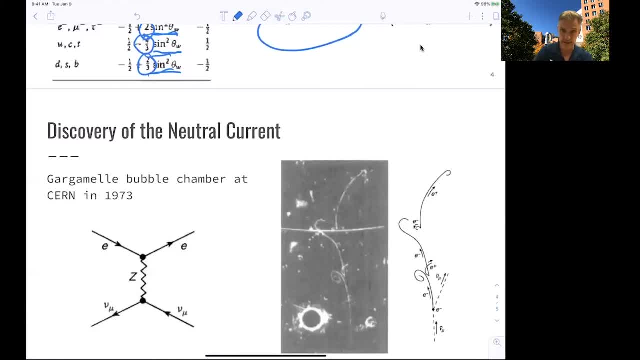 making an interaction. There's an electron And then scattering off, kicking off the electron. So what you see here is it's incoming. This is indeed an anti-neutrino kicking off an electron. See the electron here. The neutrino goes off undetected, just disappears. 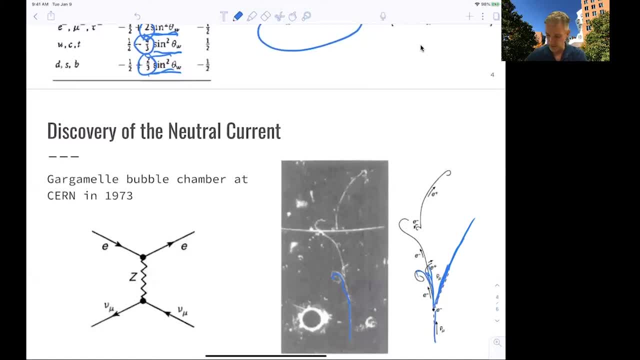 You see here the electron, And then there's also two photons. one photon here, Let's see the different color. There's one photon here causing an electron, One positron pair, And the second photon here doing the very same thing, And you can see those particles here. 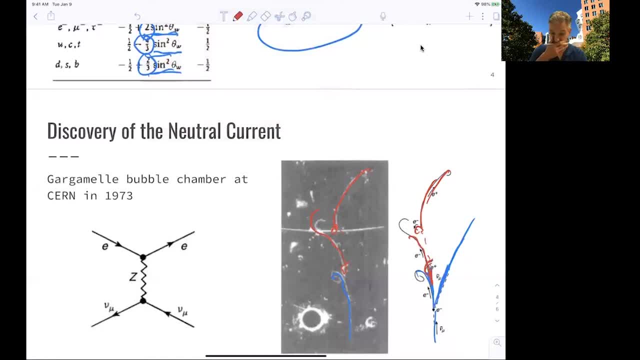 Here and there's a little ringer here as well, So this is a bubble chamber picture. We'll talk about bubble chambers very briefly later in the lecture as well, But they were extremely important and useful tools in order to illustrate, to visualize and measure particle. 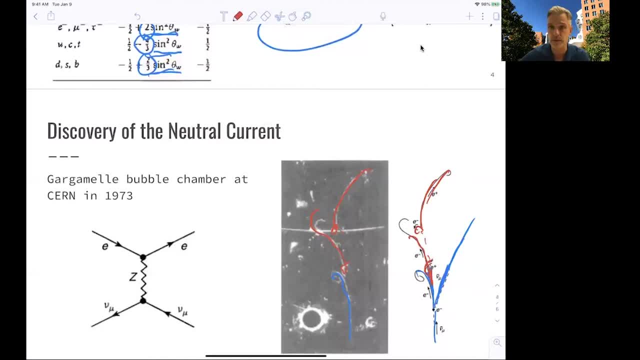 interactions. All right, So much to the introduction, And we'll continue now with the next lecture on talking about this mixture, this electroweak mixture we were talking about before. 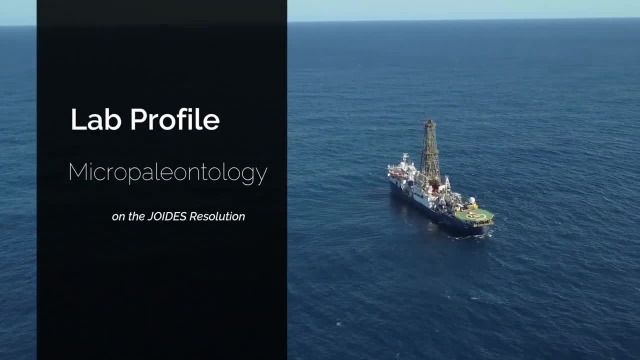 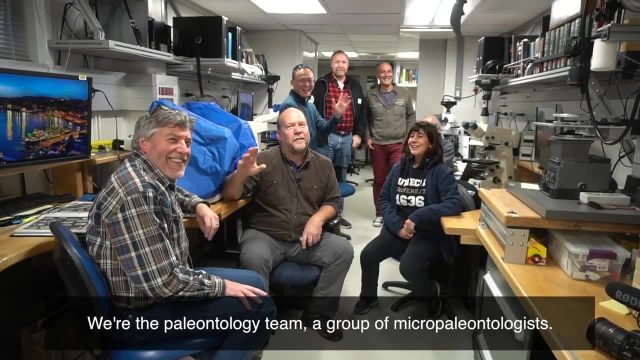 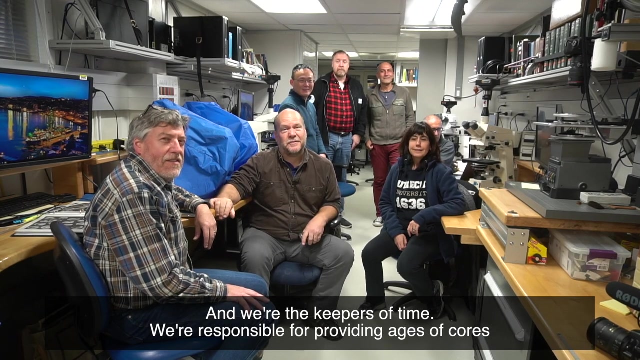 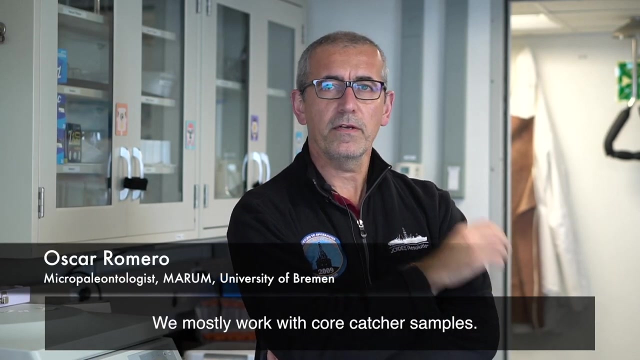 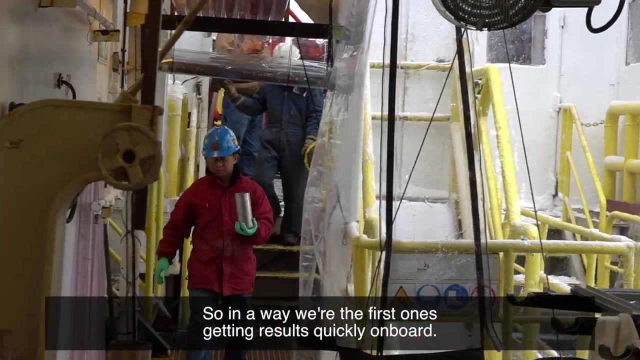 We're the paleontology team, a group of micro-paleontologists. We're the keepers of time. We're responsible for providing pages of the cores by looking at the fossils and seeing their appearance and disappearance. We mostly work with core-catcher samples, so we are the first ones getting results quickly. 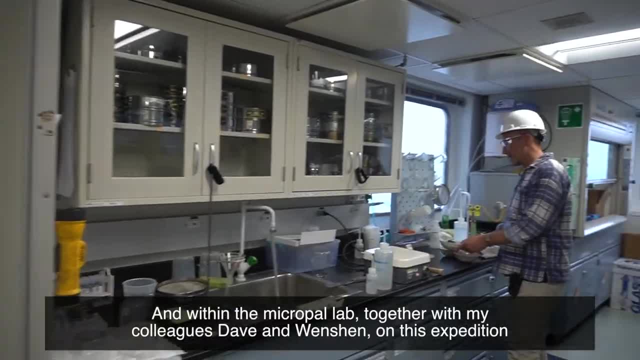 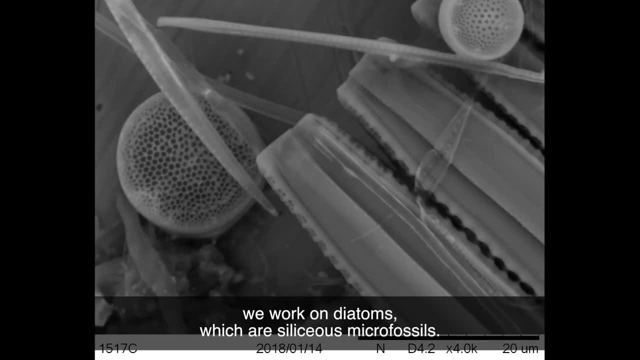 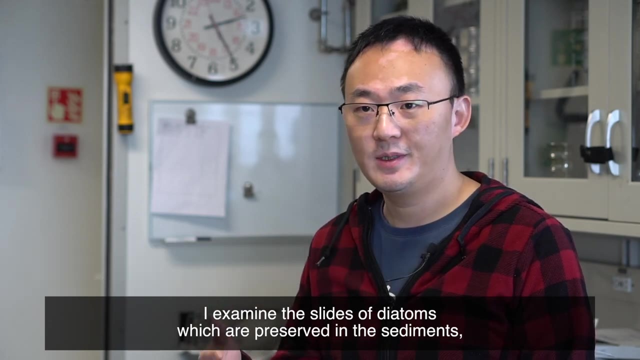 on board And within the micro-pale lab, together with my colleagues Dave and Wen-Shen. on this expedition, we work on diatoms, which are siliceous microfossils. So I examine the slice of diatoms which was preserved in the sediments which will give.